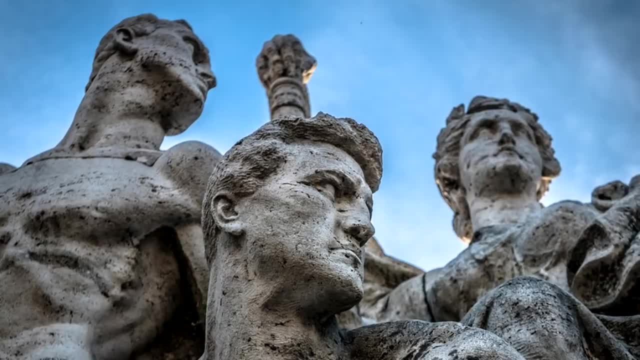 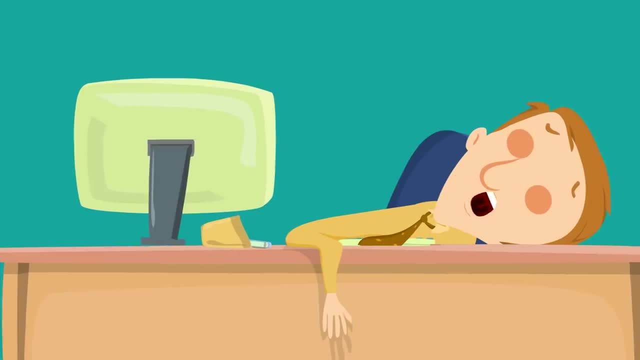 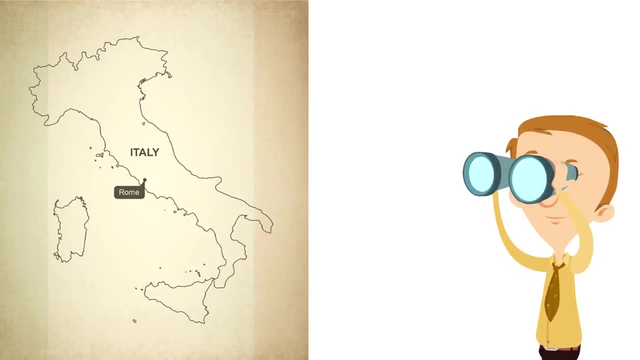 Wow, These guys look serious and, like all of our other videos, we are going to keep things fun so that you don't get bored with it, right? Because learning history should be a great time. Let's start here. Rome is a city that is in Italy. Here is the flag of Italy, the 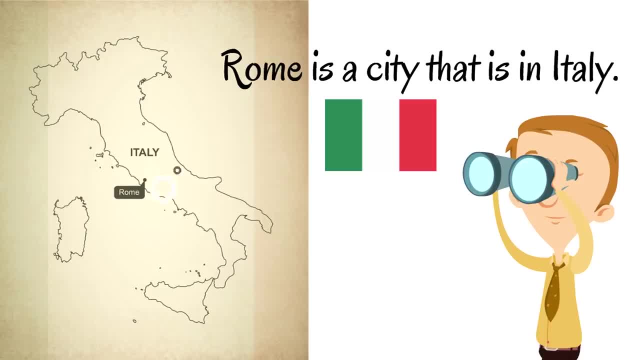 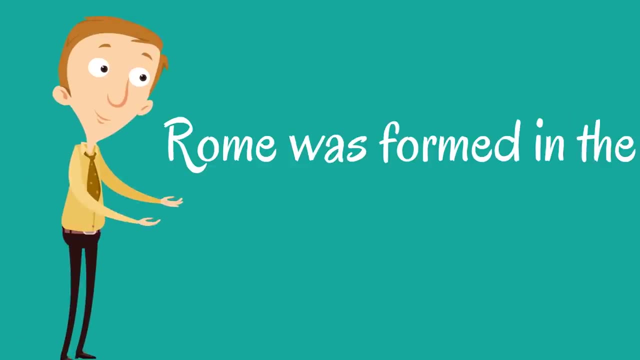 Italian flag, You could see where Rome is on the map of Italy. You can visit Rome today. today, it's an amazing place. one of the things that make it so amazing is the rich history of the city. see, Rome was formed in the 8th century BC. it was a. 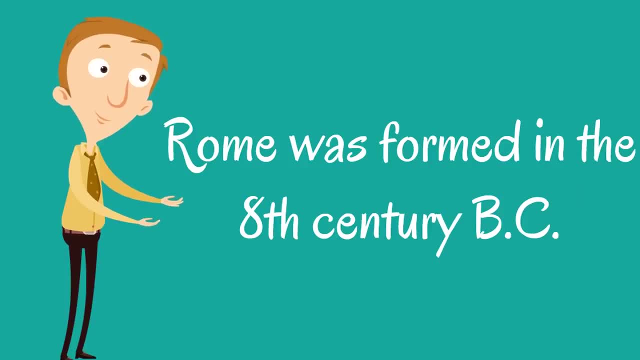 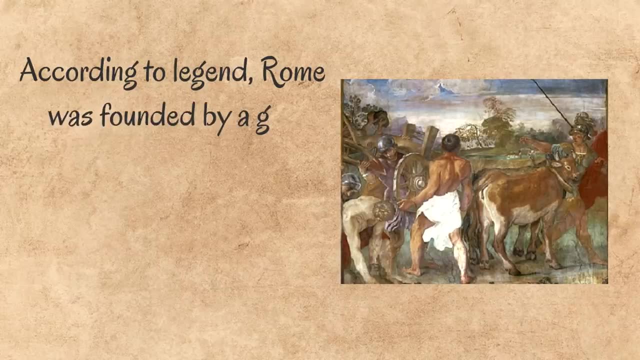 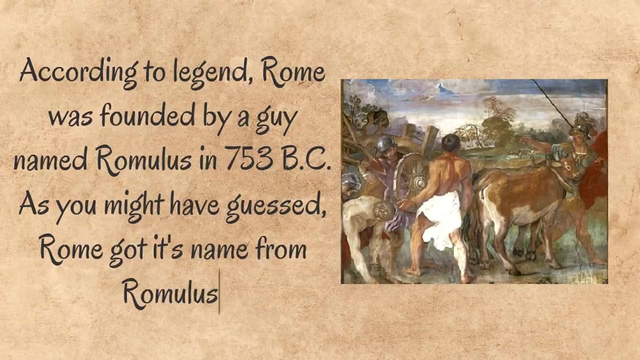 long time ago, really really long time ago, Rome as a very old city. according to legend, Rome was founded by a guy named Romulus in 753 BC. as you might have guessed, Rome got its name from Romulus. it's a cool name. you don't hear that? 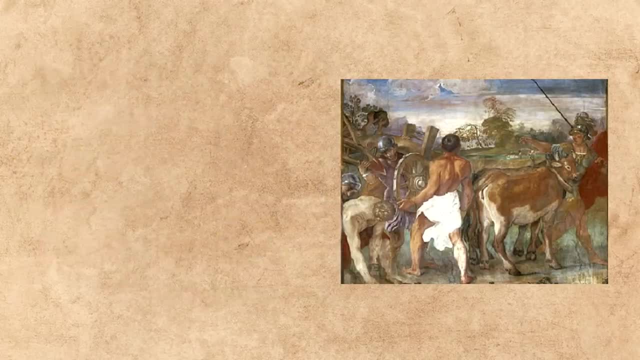 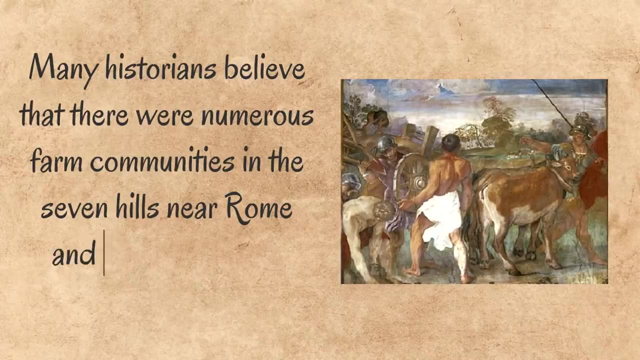 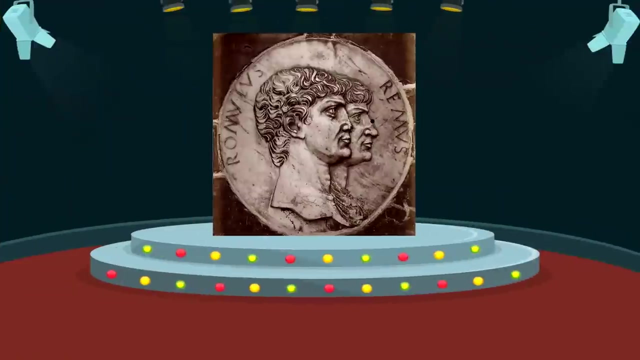 very often Romulus. well, here's the thing, though: many historians believe there were numerous farm communities in the seven hills near Rome and that they joined together to form the city. wait, that means there may have never been a Romulus. here is a coin with Romulus and his brother Remus. his brother might be. 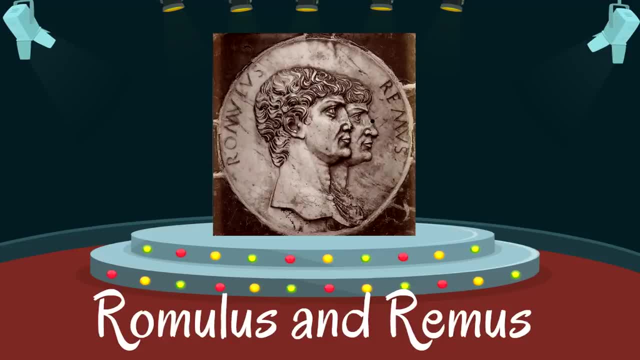 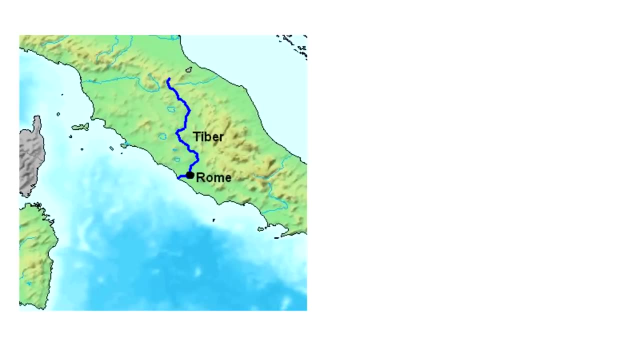 pretending to be, Romulus and his brother Remus might be pretending to be, and two, the pretend people, possibly. possibly. if Romulus was real, though, he must have been a really smart guy, because the location of Rome was perfect. first, Rome was right along the Tiber River. now, why would that be important? well, the Tiber River. 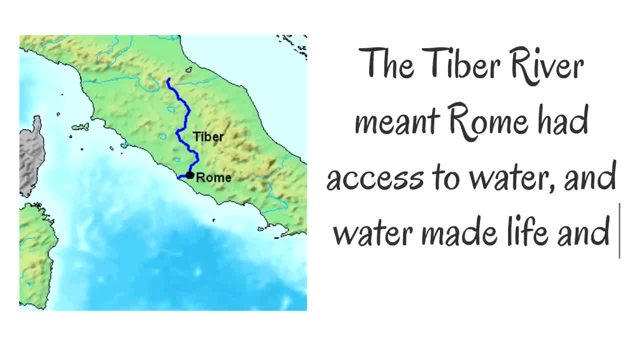 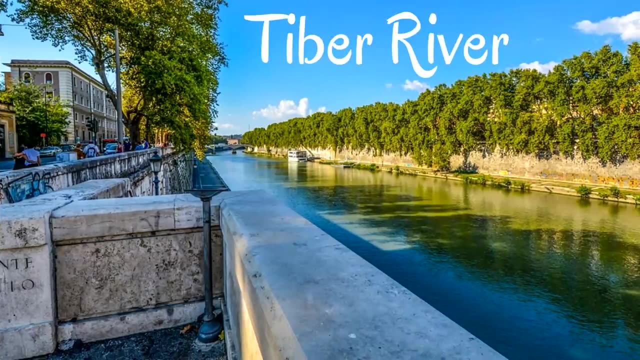 meant Rome had access to water, and water made life and civilization possible. you could see where the Tiber River is and where Rome is on this map. here is a picture of the Tiber River today. without the Tiber River, the small city of Rome would have never grown into a massive civilization. 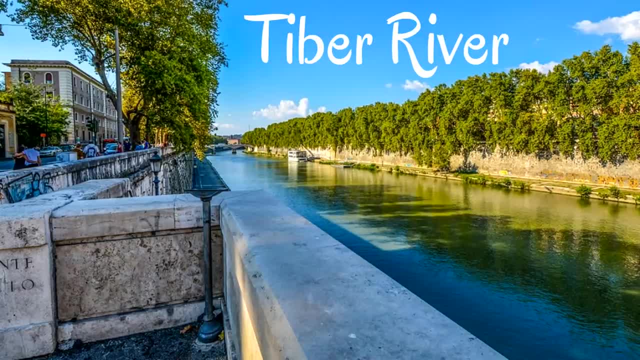 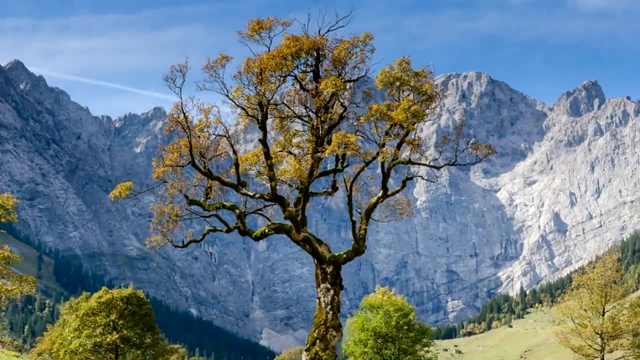 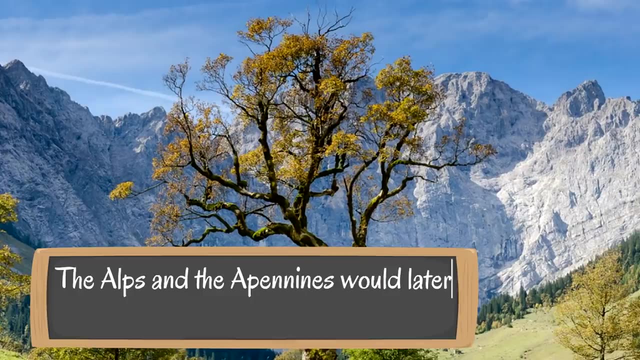 thanks Tiber River. no, no, really, thank you, Tiber. can can I call you Tiber? the second reason Rome's location is perfect is that there are huge mountain ranges that protect Rome. the Alps and the Apennines would later make invasions of Rome more difficult. not only that, Rome is surrounded by hills as well. Rome is 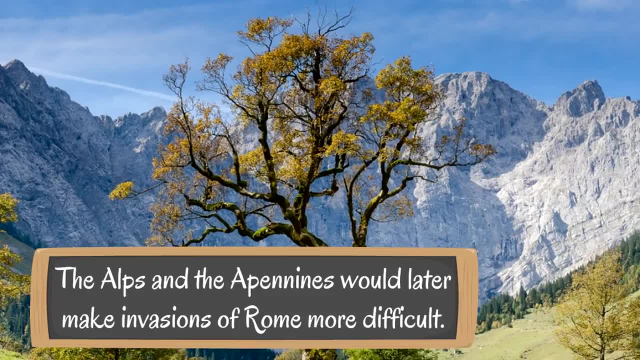 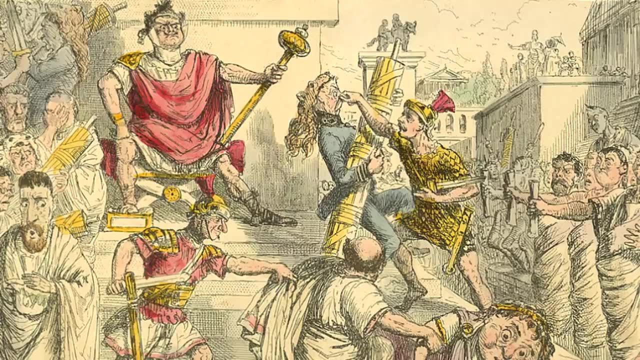 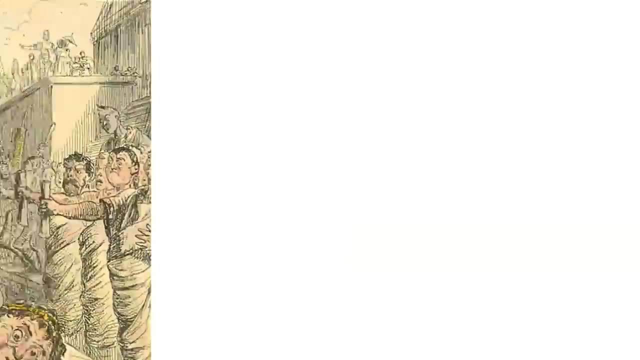 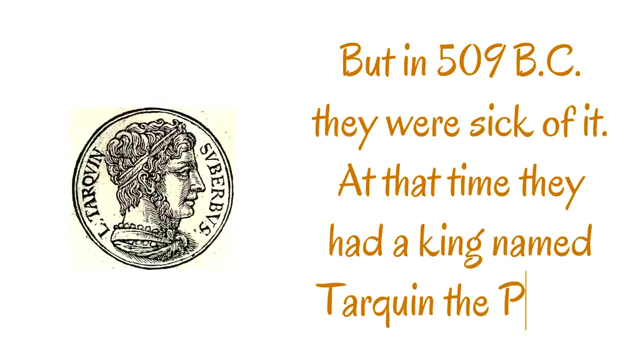 protected by natural barriers. in the early days of the city of Rome, Rome was ruled by a king. sometimes the king would be a jerk and people would be like, well, he's king, so we just have to live with this. but in 509 BC they were sick of it. at that time they had a king named Tarkwin. 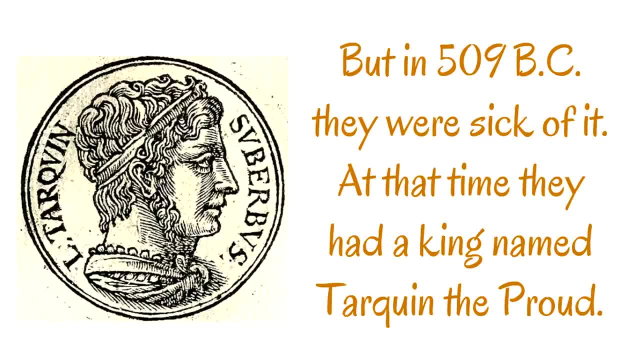 the proud, and you can see him on this coin: Tarkwin the proud. he was an awful king. he killed a lot of people, made everyone miserable and was very arrogant. that's how he got the nickname the proud. a Tarkwin the proud gotta say this. 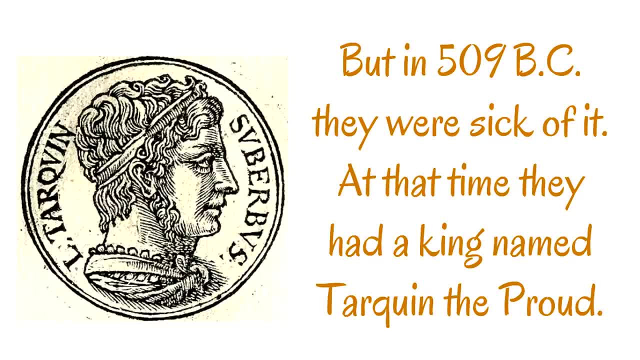 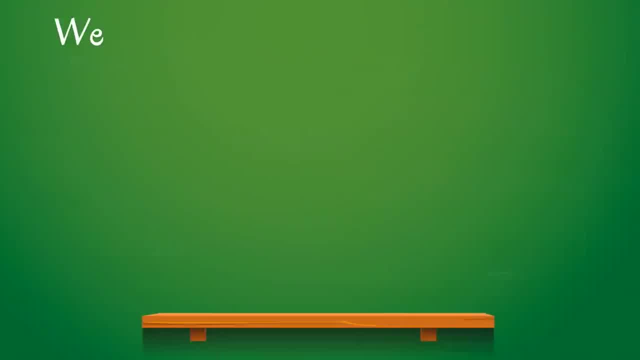 though, if this coin is accurate, while he was a terrible king, he did have good hair- that's a pretty cool hairstyle- and super vintage hair. that's all. that's all. that's all. pretty good hair. that's a pretty cool hairstyle. a, isn't it? You know Well, the people kicked him out and they decided to set up a completely. 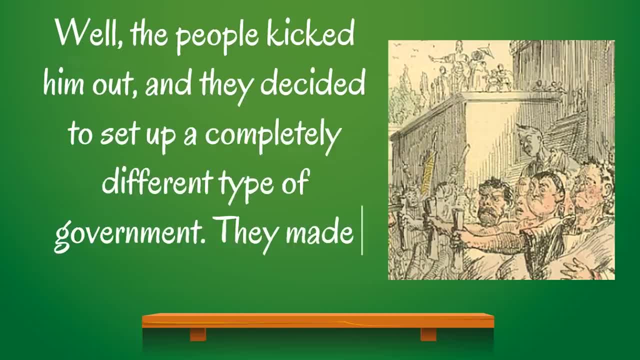 different type of government. They made Rome into a republic. You know you did a bad job as king when the place you ruled over just completely changes the government and kicks you out. OK, that's what they did, though. They kicked him out, They said you're out of here, And they said: 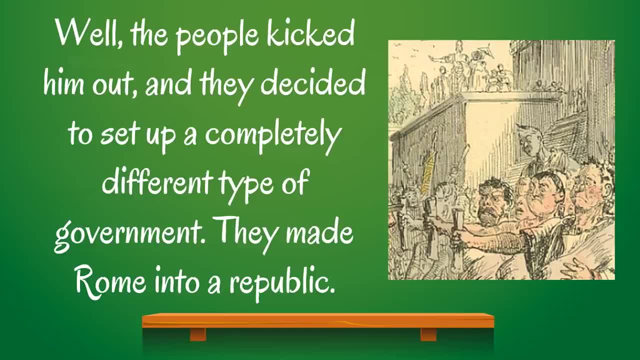 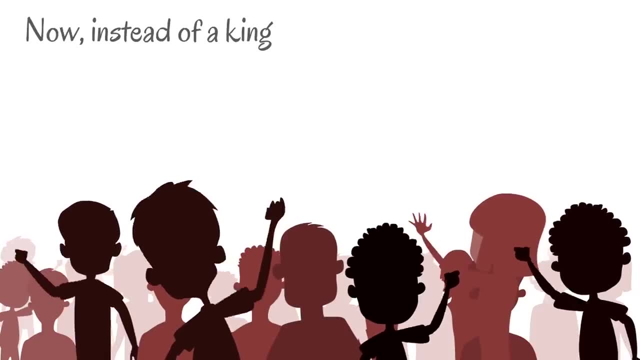 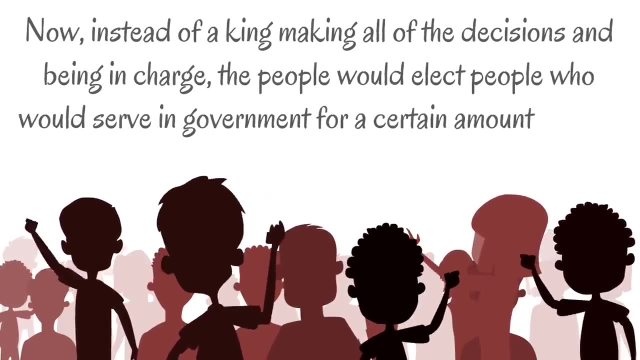 we are going to start a republic. This is going to be a republic. What a huge change that was. Now, instead of a king making all of the decisions and being in charge, the people would elect people who would serve in the government for a certain amount of. 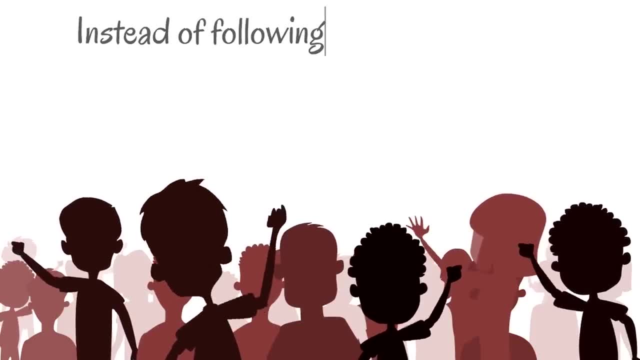 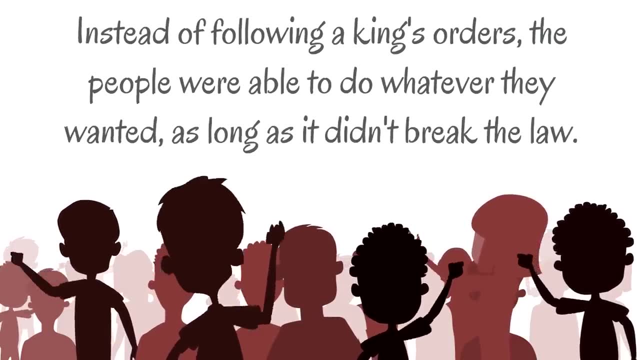 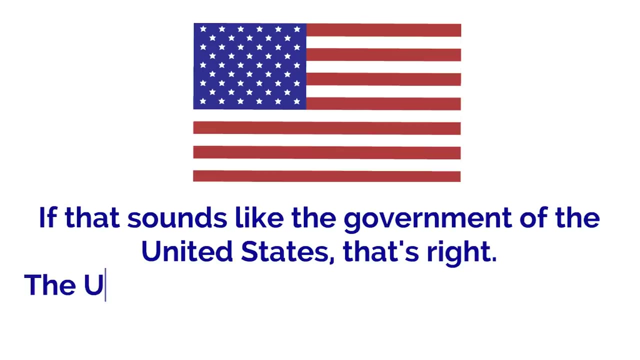 time, Instead of following a king's orders, the people were able to do whatever they wanted, as long as it didn't break the law. If that sounds like the government of the United States, that's right. The United States is a republic. Many other countries around the world are republics too. Ancient Rome was way ahead of. the curve. Rome was one of the first republics in history And under this new form of government, Rome thrived. Rome stayed a republic until 27. AD. Let's fast forward hundreds of years to meet this guy. His name is Julius Caesar. Julius Caesar. 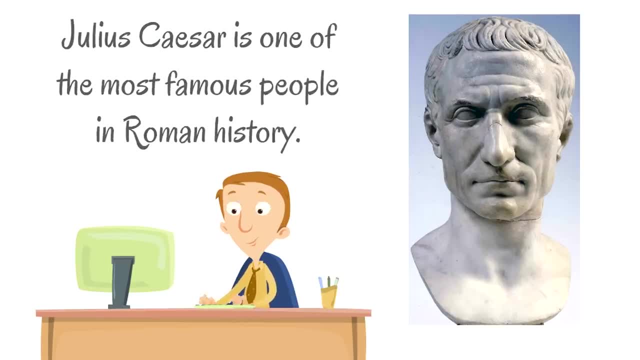 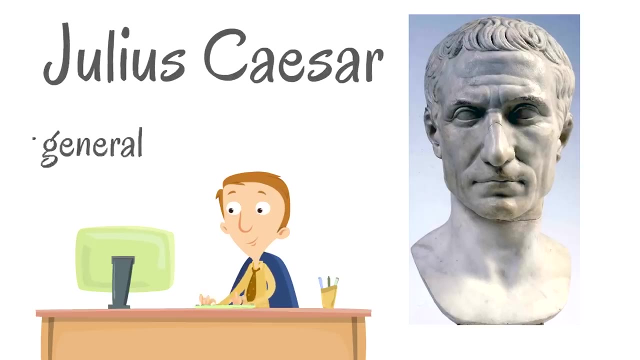 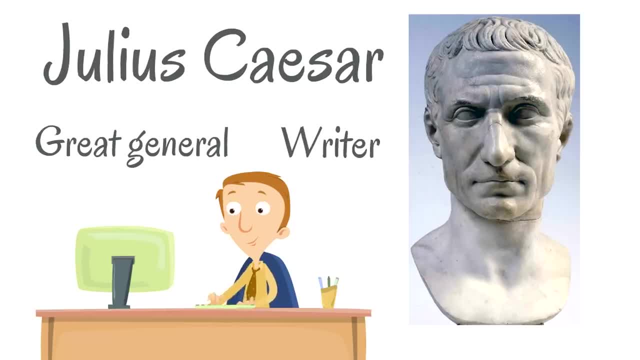 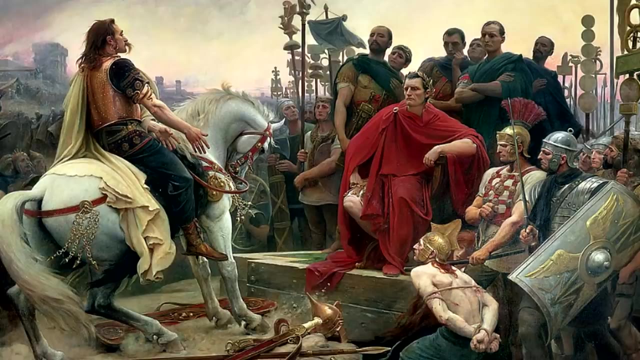 a great poet as well as a great writer. He was also a great speaker and, sł Ar Plantin, a keyricting scholar. There are Alexei V km of the writing histories of many of the battles he fought in. He was a hero in Rome and was loved by all the people. Boy was Julius Caesar until his death. 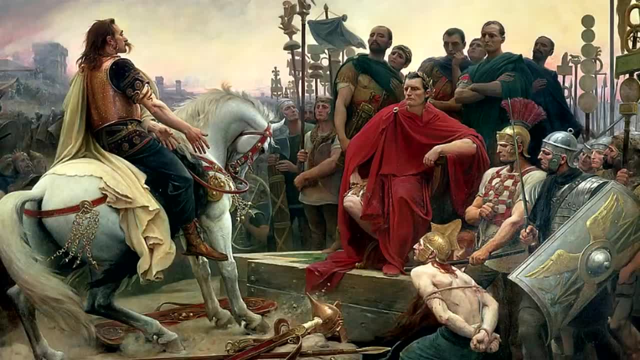 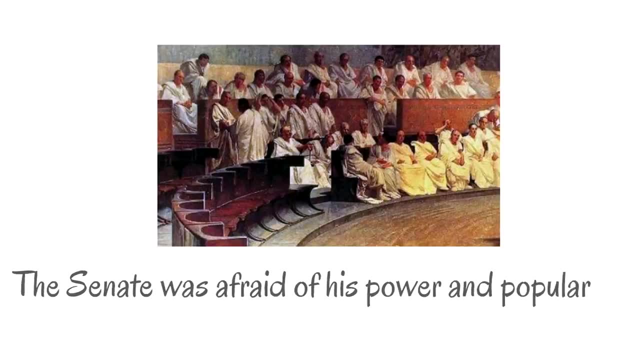 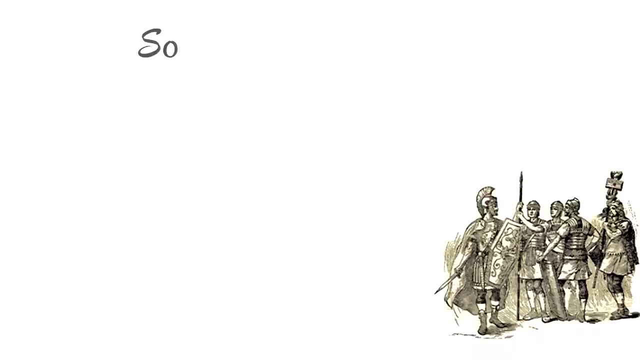 People heard of all of his victories in battle and knew that his soldiers had absolute loyalty to him. It also helped that he wrote about the battles He did a good job of always been making. senate was afraid of his power and popularity. julius caesar was a big deal. soon a civil war. 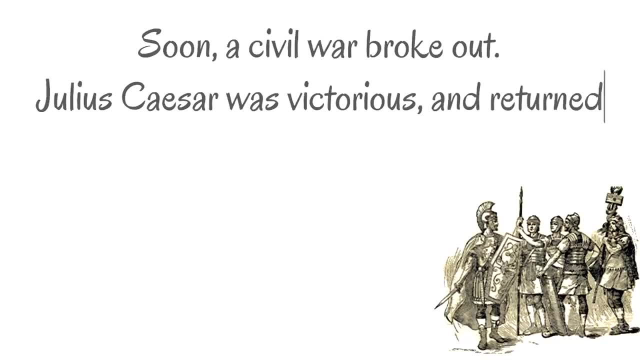 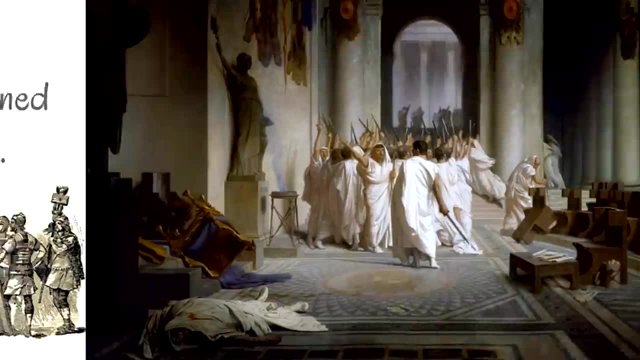 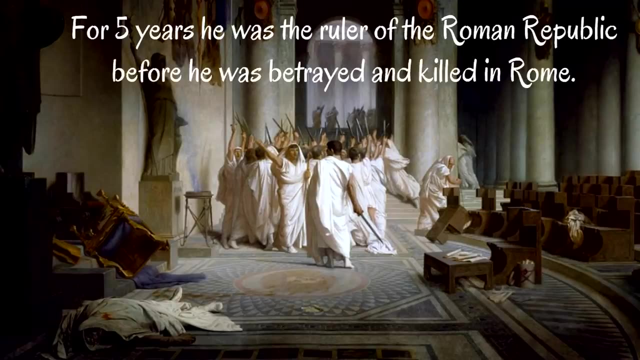 broke out. julius caesar was victorious and returned to rome as the ruler of the republic. for five years he was the ruler of the roman republic before he was betrayed and killed in rome. but ancient rome had changed forever. after julius caesar was killed, another civil war broke. 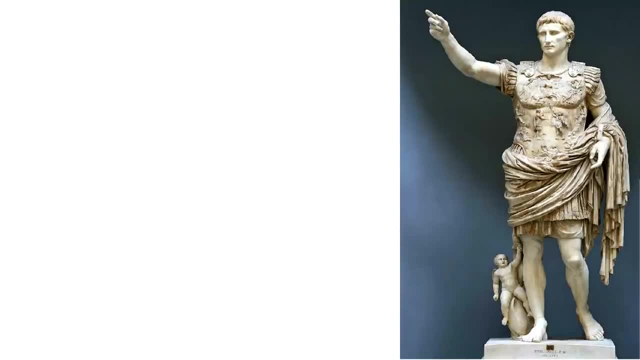 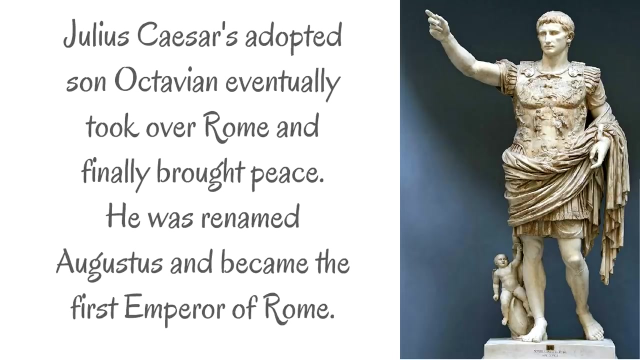 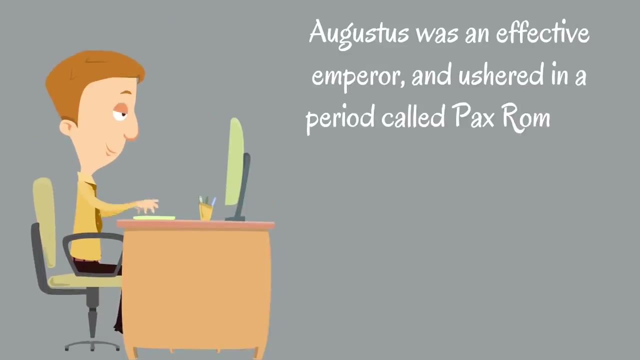 out. well, guess what happened next? julius caesar's adopted son, octavian, eventually took over rome and finally brought peace. he was renamed augustus and became the first emperor of rome. augustus was an effective emperor and ushered in a period called pax romana, where the majority of people 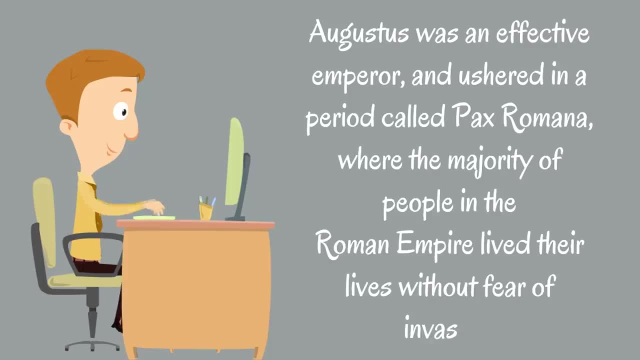 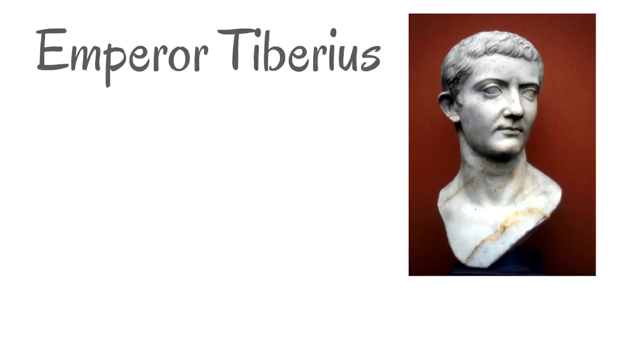 in the roman empire lived their lives without fear of invasion. pax romana means roman peace. after augustus, rome was ruled by an emperor named tiberius, the stepson of augustus. wow, all these guys are related. the republic was over and a new period called the imperial. 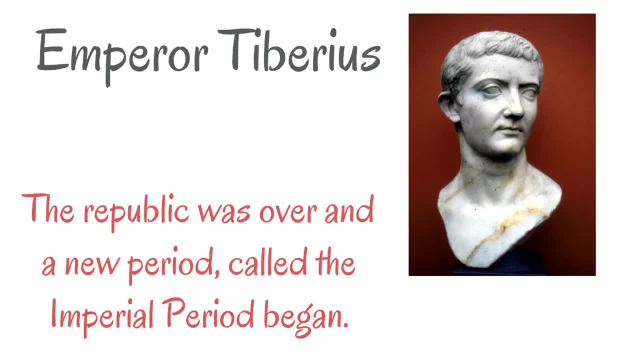 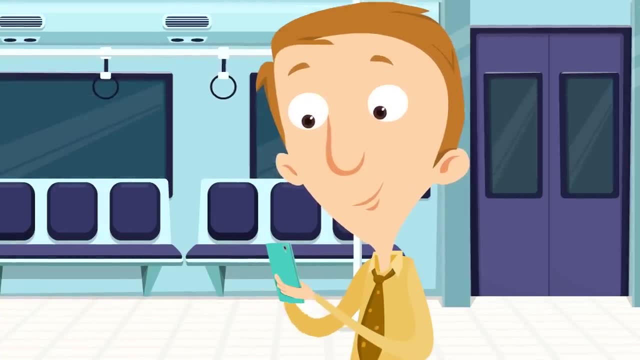 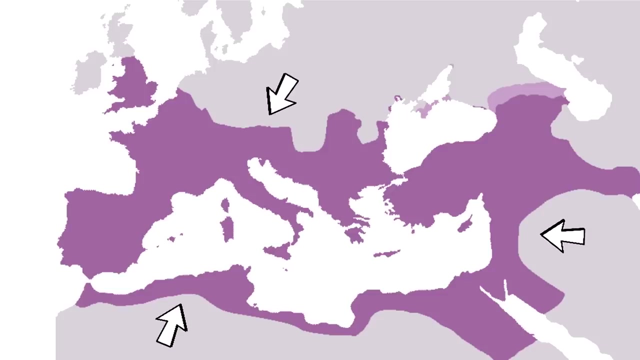 period began. wow, ancient rome went through massive changes through the centuries. now we are going to talk about the legacy of this fascinating civilization. like the size of ancient rome at its peak. see how huge ancient rome was. wow, the roman empire is colored purple. that's big. that's big. 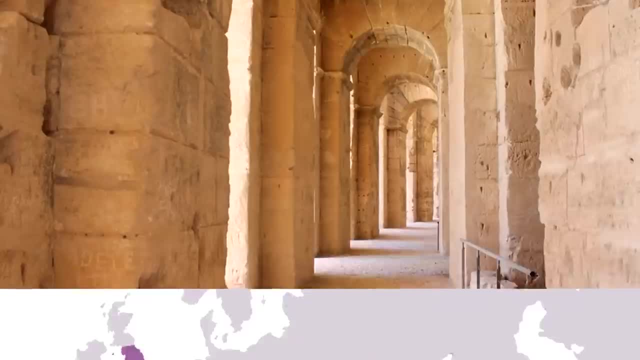 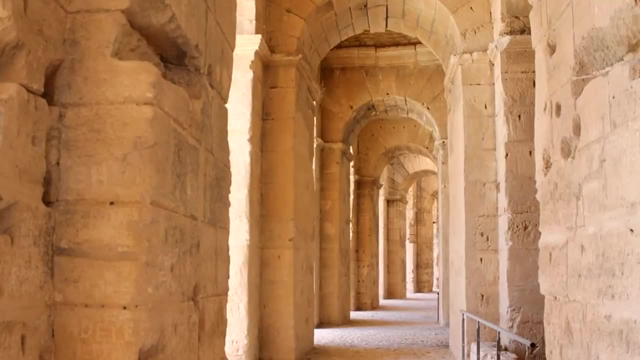 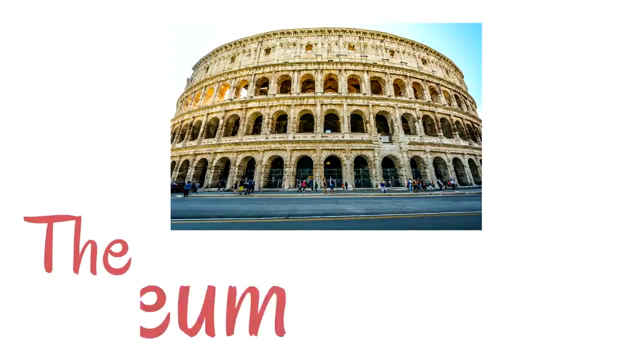 ancient rome left a big impact with architecture, with many of their structures still surviving and standing today. probably the most famous example is the coliseum. the coliseum was a massive amphitheater in the city of rome that still amazes people today. over 60 000 people could watch sports and events. 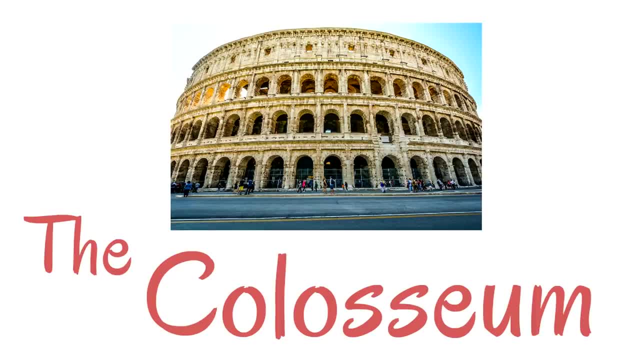 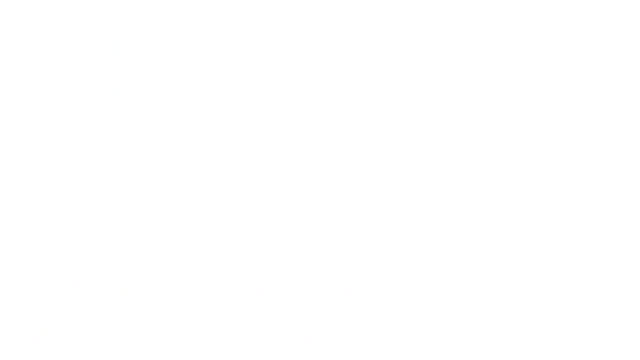 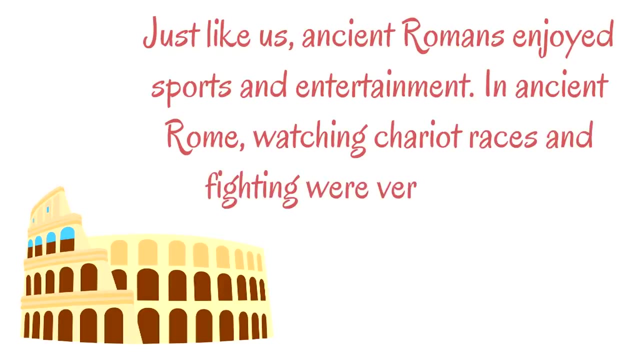 in the coliseum. this is what the coliseum was made of: sports and events in the Colosseum. just like us ancient Romans enjoyed sports and entertainment, in ancient Rome, watching chariot races and fighting were very common. the fighting, though, would be very violent. unfortunately, many people 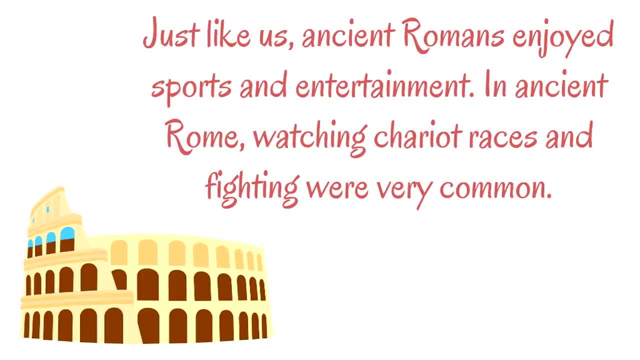 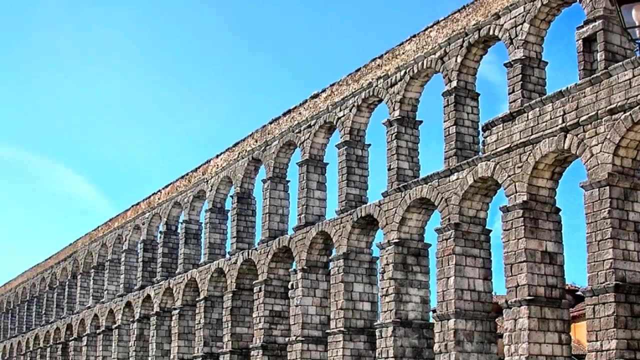 lost their lives in the Colosseum and to us that type of fighting doesn't even sound like a game. but in ancient Rome people filled the Colosseum to watch fighters called gladiators fight it out. this is cool. ancient Rome is also known. 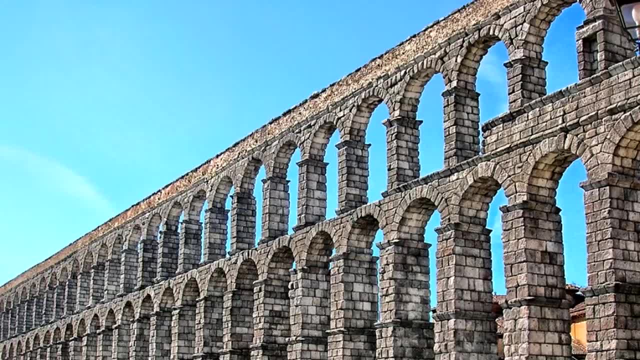 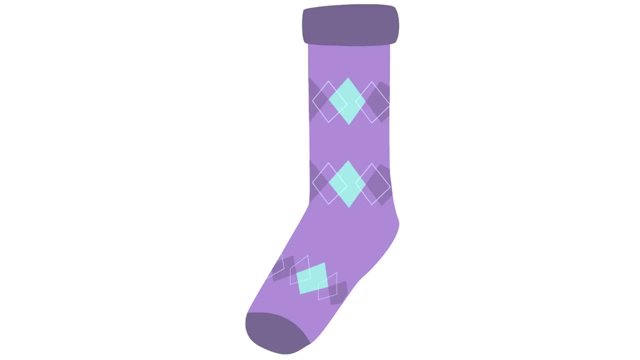 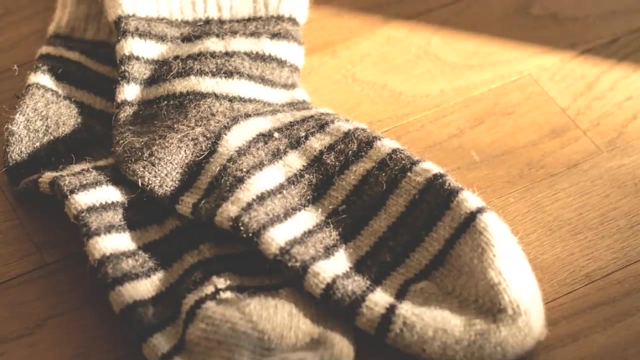 for having water systems and aqueducts bring fresh water to different places. ancient Rome also had sewers to dispose of waste- very important. these advancements helped many people live a better quality of life. ancient Rome also invented socks. seriously, seriously, okay, next time you wear socks, just think, wow, thank you ancient Rome. these are really cool how.